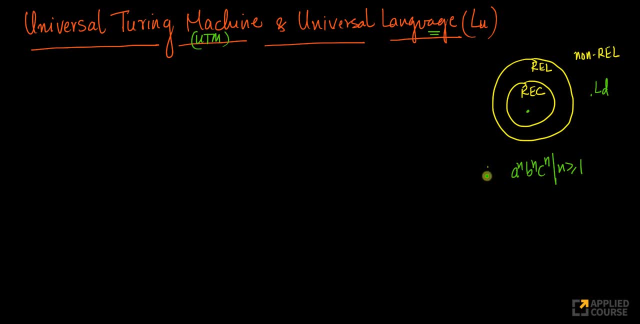 than equal to 1.. So this language, this language we know, this language we know is recursive. So we know this language to be recursive. Are there languages here which are recursively enumerable but not recursive? Look at this: Are there languages which are recursively enumerable but not recursive? We have seen 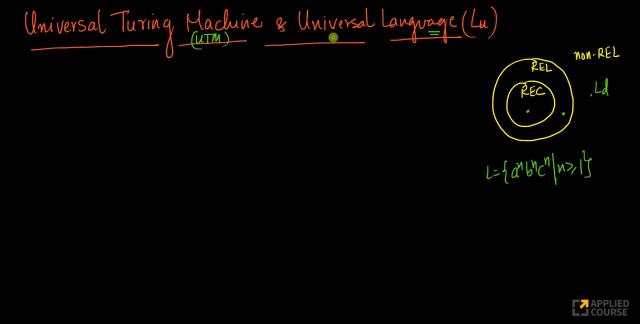 a non-recursively enumerable language. Now we will. we will first understand the Universal Turing Machine concept. We will also understand what is Universal Language, And in the next couple of videos we will show that LU is a recursively enumerable language, but not. 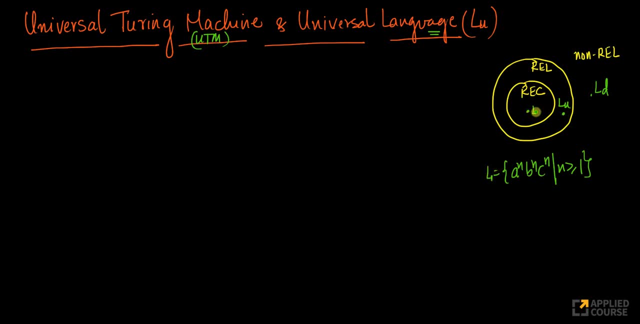 recursive. So let us call this language as L1.. This L1 is a recursive language. Now we have languages across the spectrum. We have seen recursive languages. We will learn, we will. I will prove this to you in the next couple of videos. First, let us understand. 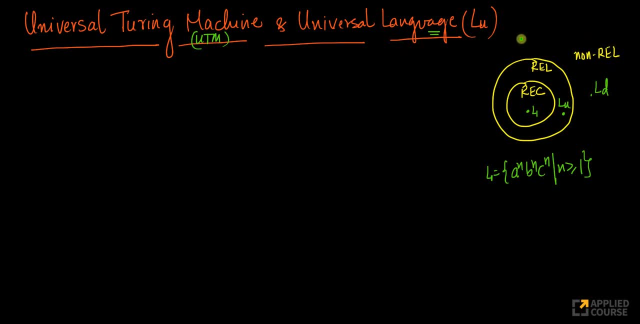 what UTM is and what Universal Language is. But I am giving you a big picture overview here. We have learned that LD is a non-recursively enumerable. Let us also show that LU is a recursively enumerable language. And when I prove that LU is a LU, the Universal Language. 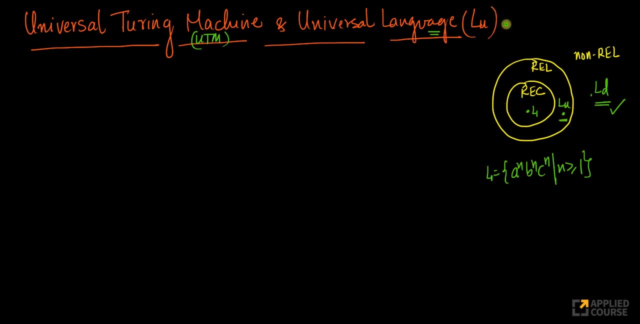 is recursively enumerable but not recursive. This will also lead us to Halting Problem Again. I will define Halting Problem much more formally here and I will also prove this Again. we have been talking about Halting Problem from the very first video on Theory of Computation, Right. So this basically says: given a computer, 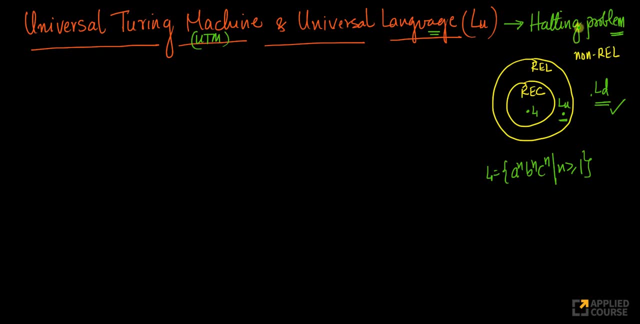 program and some input. would that program halt or not? Right, We will. we will come to this. So over the next two to three videos, these are the topics that we will cover. But first let us understand what is a Universal Tuning Machine. So okay, before we go there, 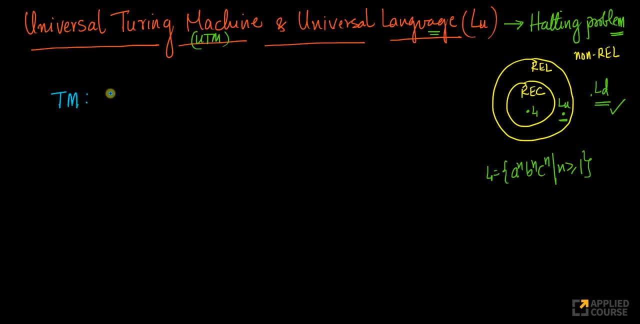 let us understand. what is a Universal Tuning Machine? Right? So you can think of each Tuning Machine. You can think of each Tuning Machine as a program. Right, Each Tuning Machine is a program. For example, I can construct a Tuning Machine for this. What does that? 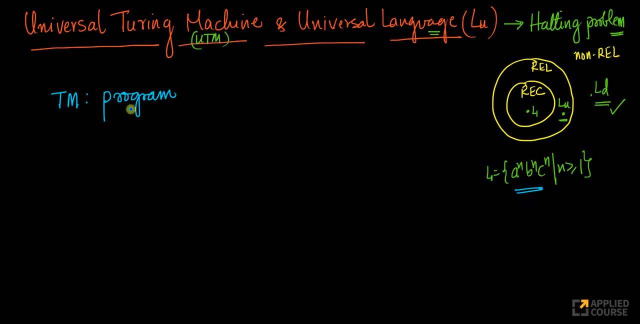 do That gives me. you can think of it, if you think about from the world of programming. you can think of Tuning Machine as a program And if I give a word, if I give an input, if I give, let us say, AABBCC, this program can tell me, this program can tell me whether 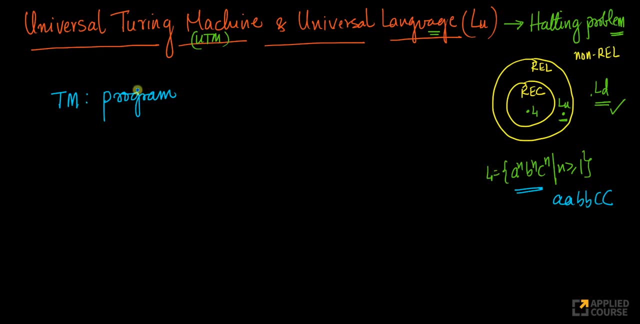 this word belongs to this language, or not? Right That is. that is one way of thinking about a Tuning Machine. So now, Universal Tuning Machine. now, the word Universal here basically means a Universal Tuning Machine behaves like a general purpose computer. What? 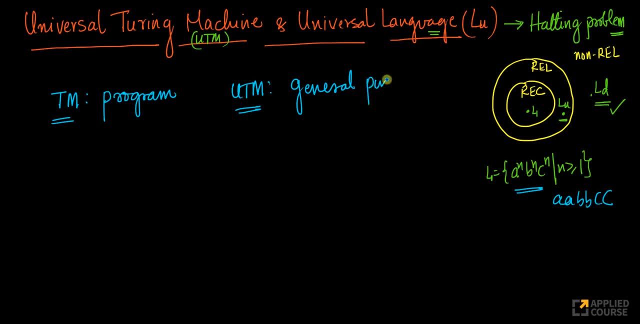 how does that? what, what? how do we actually use a computer? Okay, It uses, it works like a general purpose computer. So what happens in the real world is to a general purpose computer. you give a program, Right, You give a program and you give inputs And the computer 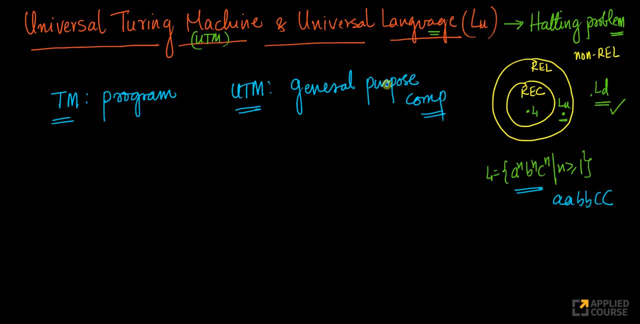 takes the program and the inputs and generates outputs. That is what it does, Right? So imagine if there is a Tuning Machine. Again, this is a. this is a. this is a rough analogy that I am giving you The exact mathematics of the exact details of Universal Tuning. 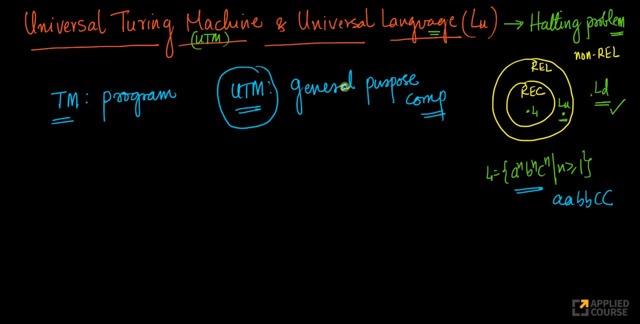 Machine. we will learn in a little while, But this is the intuition behind it. You can think of Universal Tuning Machine. So think about it like this: Right, A Universal Tuning Machine is also a Tuning Machine. Remember, a Universal Tuning Machine is a special type. 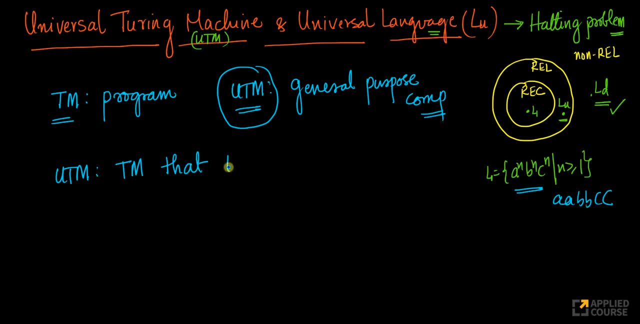 of Tuning Machine that takes it is a Tuning Machine that takes a Tuning Machine code, that takes a Turing Machine code. What is a Turing Machine code? A Turing Machine code is nothing but the binary strings. We have seen this Right. I can encode a Turing Machine using a binary. 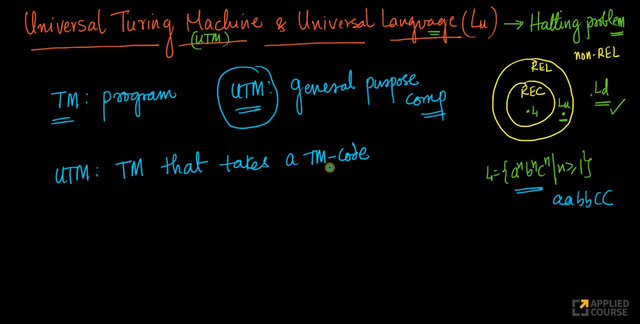 string. A Turing Machine code is nothing but the binary string, This Turing Machine code, or the binary, the binary representation of a Turing Machine. It takes a Turing Machine code as input and and it takes a word as input. as inputs, It takes two inputs: It. 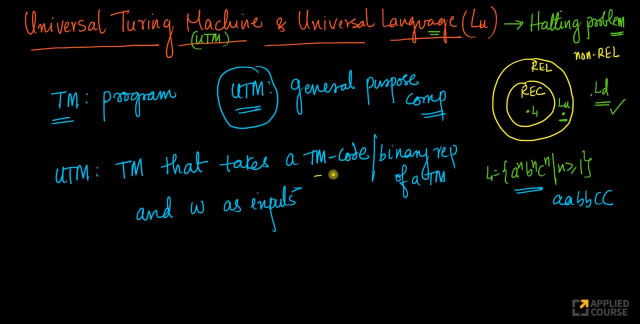 takes a turing machine code, Right. So it takes two inputs. The first input is the Turing Machine code itself. You can think of the Turing Machine code as the program And it takes a word also as input And what it does now It takes both. Remember, UTM itself is: 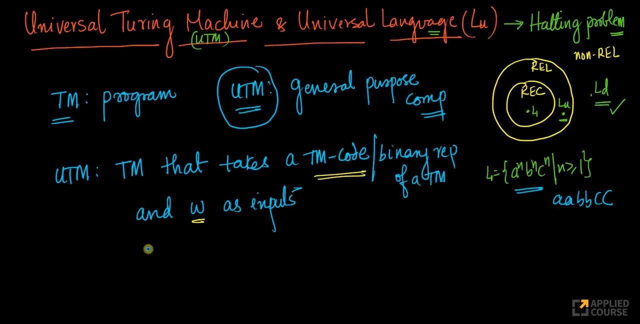 a Turing Machine, but it is a special type of Turing Machine And this Turing Machine. So you take these two inputs and it accepts. it accepts the inputs, t accepts this input, It accepts the inputs, It accepts the inputs. The input words are also Turing machine. So in each machine you 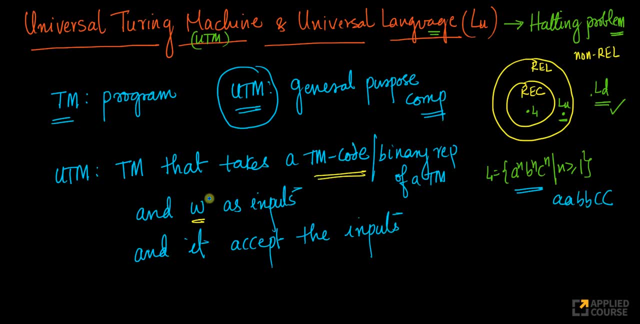 word. right, the input word consists of turing machine code and the word that we want, that that we want- and a word. okay, i'll tell you why this, how this word and turing machine are related. right, so it's a turing machine that takes a turing machine code and a word as inputs. 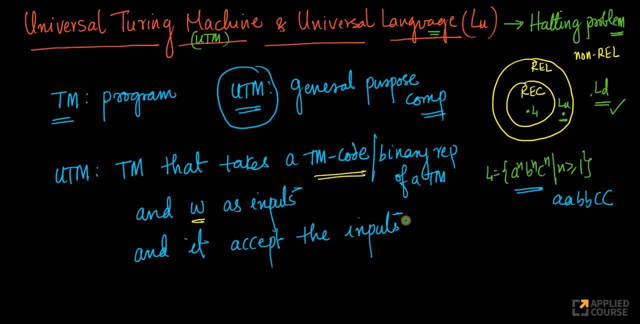 and it accepts the input word. it accepts the inputs or input word or input word: if and only if, if and only if, if and only if this word w will belongs to the language accepted by this turing machine. so let's call this turing machine as m, right? so let's call this turing machine as m. 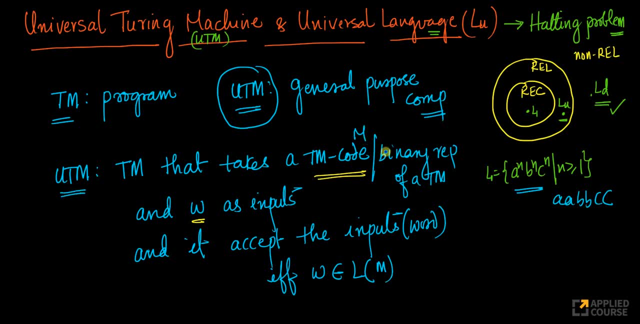 right. so universal turing machine takes a turing machine code m as input and it takes a string w as input. it is taking two things as input and it accepts. it accepts the inputs if, and only if, this word belongs to this turing machine. so in a. in a nutshell, this universal turing machine is executing this turing machine. 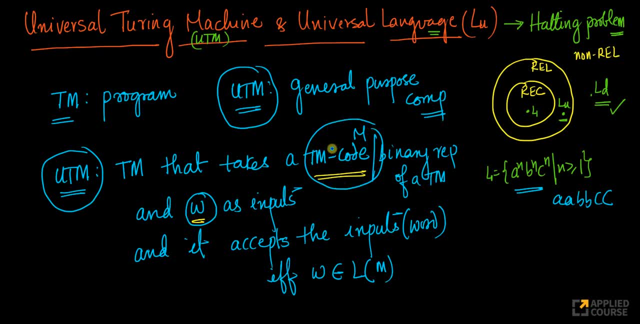 and it is verifying whether this turing machine will accept this word or not. that's what it does in a nutshell. that's what it's doing now. your question should be: what? how do we input? see, there are two inputs here. right, there is a turing machine code. 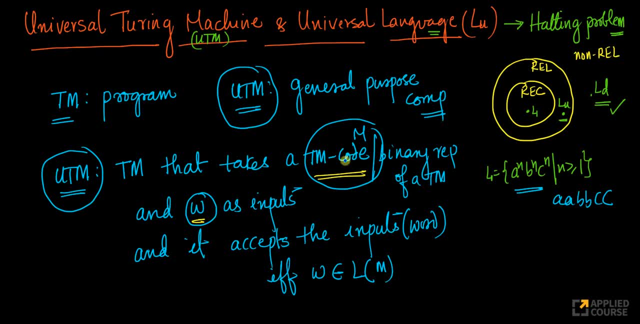 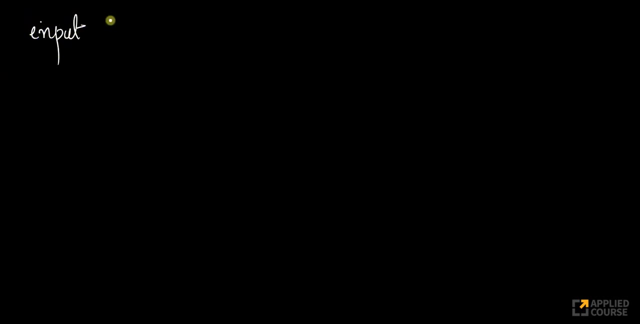 and there is a word as an input. how do i input both of them as inputs, right? so we'll come to again. this is the big idea. i'll explain you how the whole, how the whole utm works internally. just just take in a few minutes, you'll understand this, right. so how do we input? so input word input to a utm. 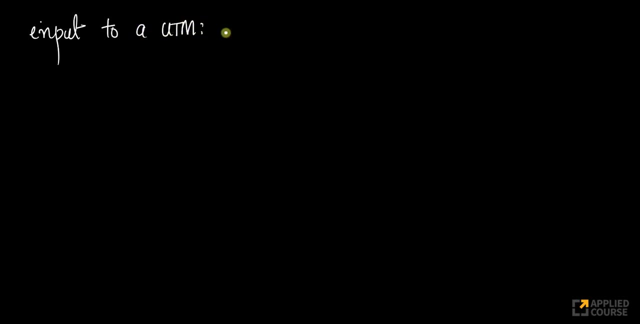 how do we input to a universal turing machine? very simple: you take the code for you take the code, the binary code, right? you take the binary code. so i'll use the words binary string and binary code, right? i'll take the code for m: right? this is, this is a binary string. remember that this. 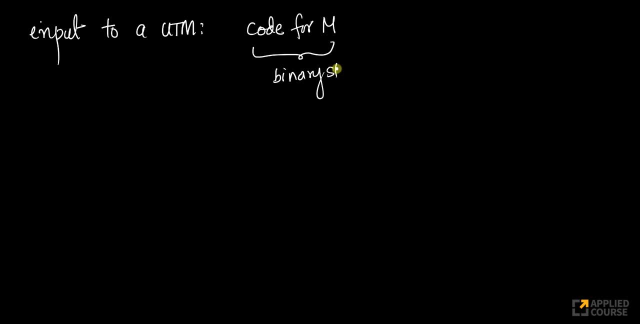 is a binary string. this is a binary string. this is the binary representation of your machine m. then i'll place three ones. i'll place three ones here because in the code for m you will not encounter three ones anywhere. you'll encounter a one or you'll encounter two ones. look at this: how? how did we define the whole binary representation? 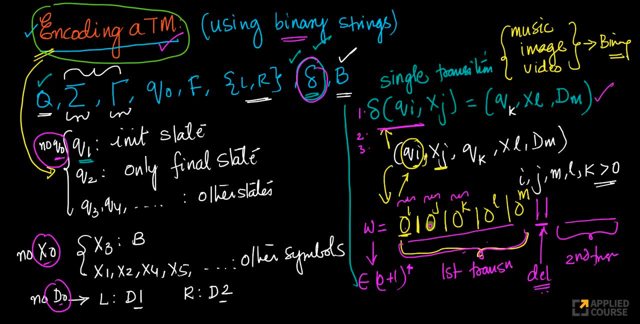 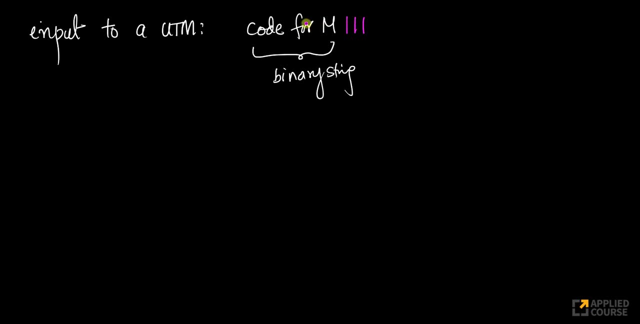 of turing machines, you have ones separating each of the symbols in a single transition. two transitions are delimited or separated using two ones. you will never encounter three ones, right? so? so what I'll do now is this: so, because I want to give the code for M. 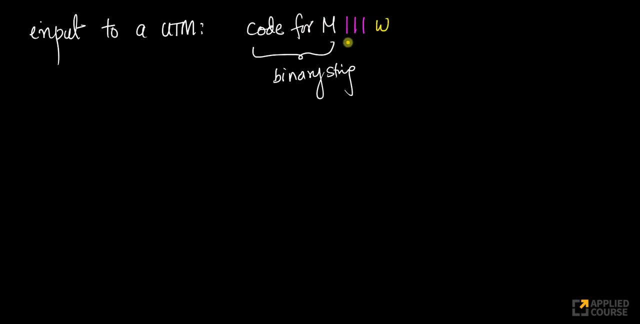 and now I'll also give the word itself. so this triple one here. this triple one is working as a delimiter or a separator. this is working as a delimiter or a separator, or a separator between the code for M and the input itself. this is how I input to a Turing machine or to a UTM way: UTM- I need to send two input. 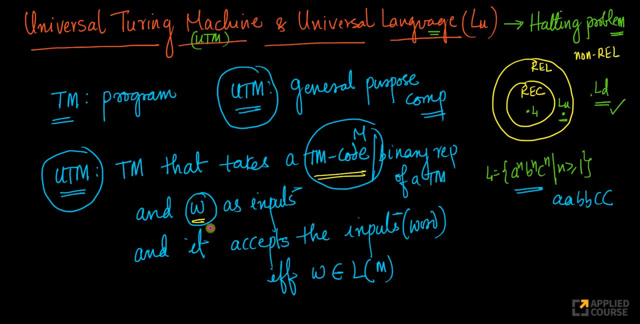 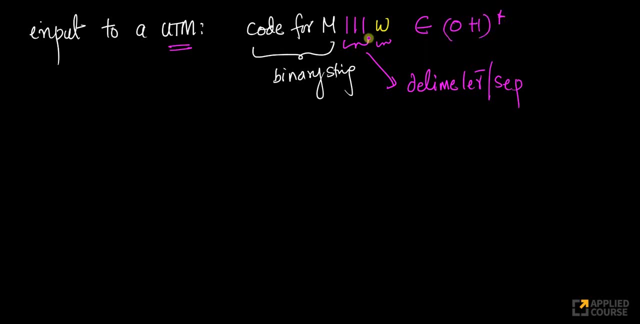 strike. one input is a Turing machine code itself. the second input is the word itself. this is how we input it. if you notice, this belongs to 0 plus 1 star. this is also a binary string, right as long as your word itself is a binary string. here, I'm assuming, by default. from now onwards, I assume, that the word is a. 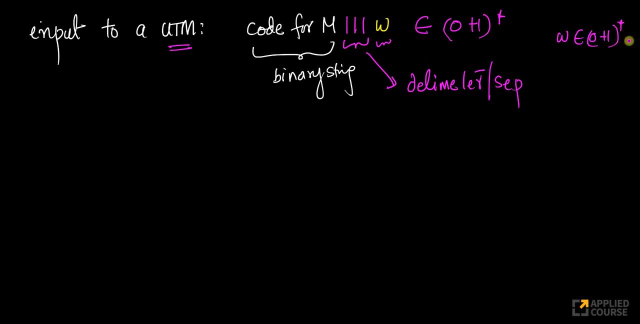 binary string, unless stated otherwise. okay, so I'm assuming that the word is a binary string. the code for my Turing machine M itself is a binary string. so this whole thing is a binary string, right? so this is how I give my inputs very simple. now I can define my, so look. 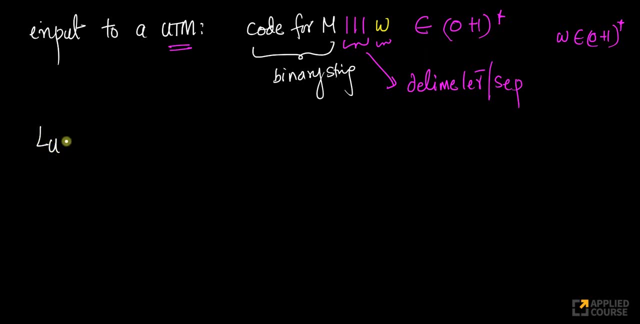 at this. I can define my language, you. look at this, I can define my language, you, or the universal language, as follows. now take: so these are all binary strings, right, so this is a set of strings. look at this, this is a set of strings. okay, it is. let me write it in English. I think that's better, okay, okay, so let me write. 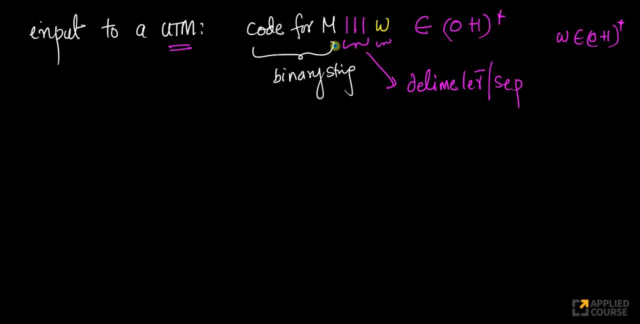 it slightly differently so that it becomes easier for you to grasp this concept, right? so now. now these are the inputs to a U universal Turing machine on some inputs, on some input words right, on some. on some input words. right, you don't have two inputs now, you have a single input. 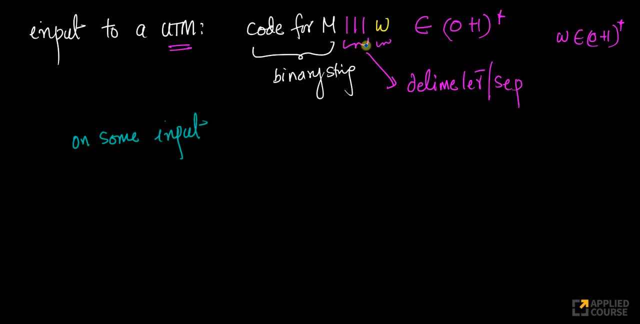 word, because I concatenated the two inputs using a delimiter. on some inputs, your universal Turing machine will accept them. universe. on some inputs, universal Turing machine accepts. on others because it's a Turing machine, because it's, at the end of the day, UTM is also a TM right. UTM is for. 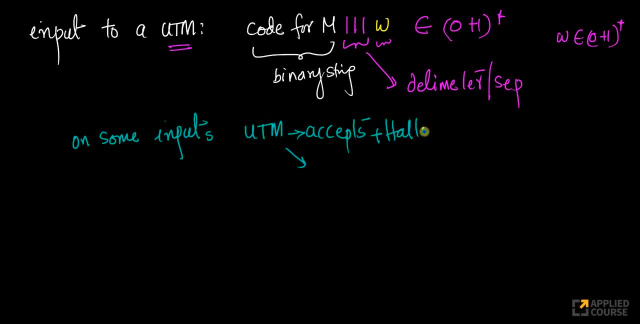 UTM is for some it accepts and holds right accepts. some it accepts and holds right. accepts. some it accepts and holds right accepts. accepts basically means final state plus accepts basically means final state plus accepts basically means final state plus halt. that's what accept basically means halt. that's what accept basically means. 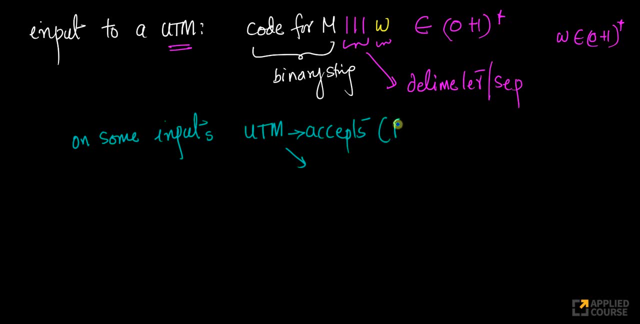 halt. that's what accept. basically means right except. basically means final state right except. basically means final state: right, except. basically means final state plus final state plus halt, or it rejects plus final state plus halt, or it rejects plus final state plus halt, or it rejects. there is another possibility: it rejects. 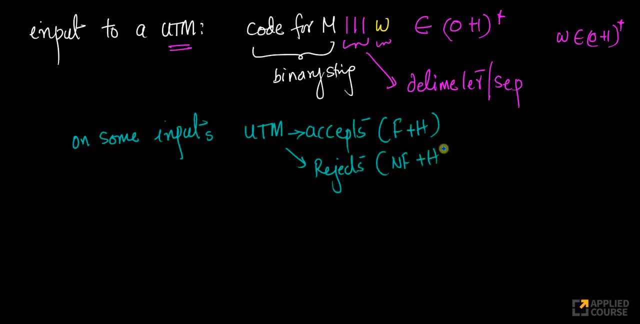 there is another possibility it rejects. there is another possibility it rejects: which means non final state plus halt, or which means non final state plus halt, or which means non final state plus halt, or it goes into an infinite loop or it goes. it goes into an infinite loop or it goes. 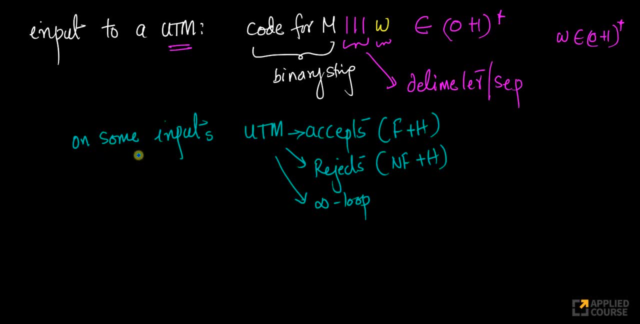 into an infinite loop, right? So all the words, all the inputs, all the inputs on which your UTM accepts, okay, let us call that language as LU. So LU is nothing but the language accepted by U, where U itself, where U itself is a universal Turing machine, If I call universal Turing. 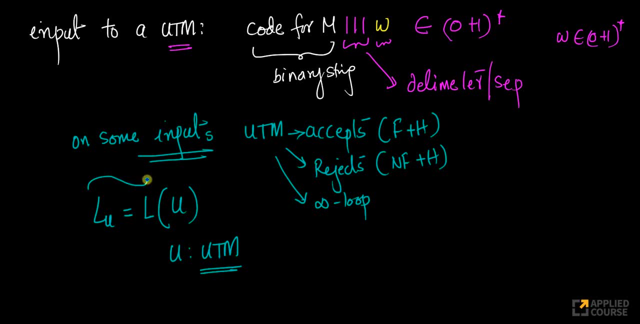 machine as U. LU is the language accepted by U, which means it consists of all the words, all the binary words, such that when I interpret this binary word as a code for a Turing machine delimited by triple one and a word, if this word is accepted by this Turing machine M. 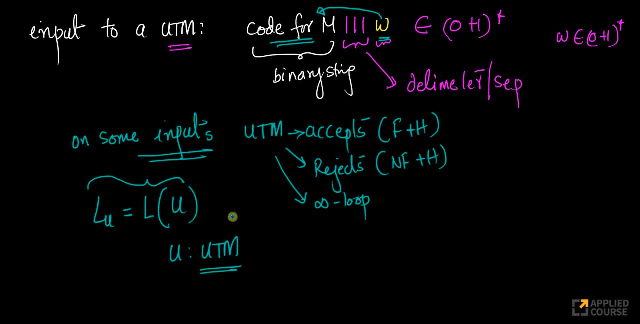 then I will accept it even in the UTM, right, Then that word, then this whole binary word is accepted by the UTM. That is how I am defining. this language is called as a universal language, And this language is called the universal language. 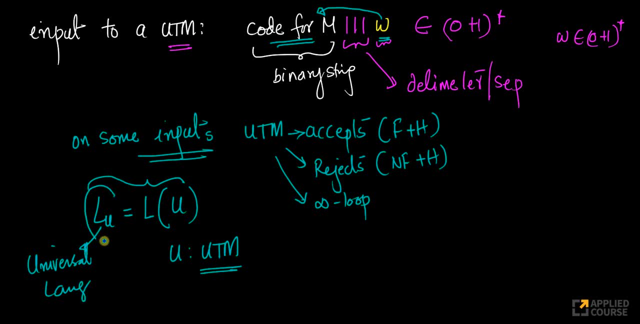 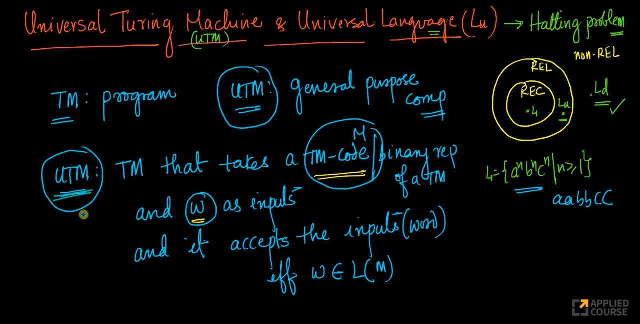 Now the big thing is that when I interpret this binary word as U, I will accept it even in the big question. here is again: we will understand the properties of universal language over the next couple of videos. But the big question here is: how does the UTM work, How does the UTM itself? 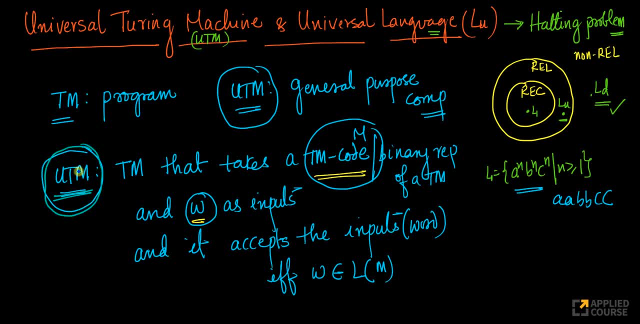 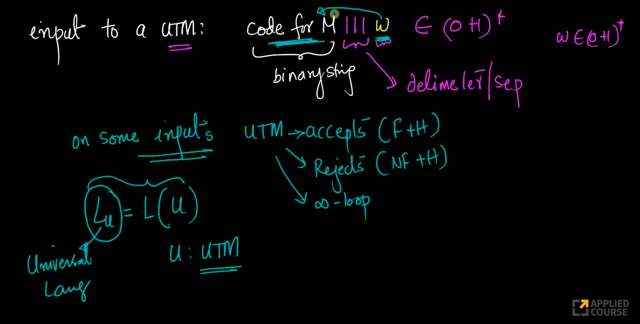 work Because? because what should the UTM do? if you think about it? The UTM takes the code for M. UTM also takes the word. Now it has to simulate exactly how this Turing machine works on this input And on this input. if this Turing machine goes to a final state and halts, then the UTM 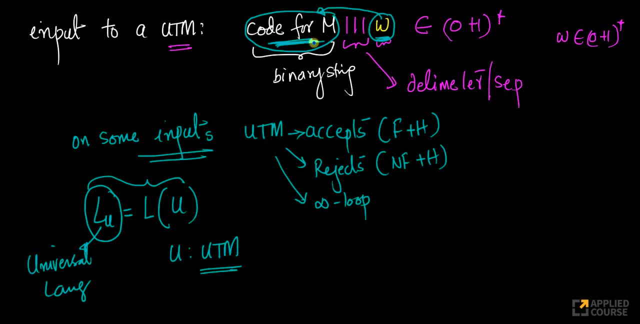 should also be able to do the same thing. So if this Turing machine goes to a final state and halts, then the UTM should also say: yes, this word is accepted by this Turing machine, Else not. So that is how it has to work. Now let us try to see how to actually how this UTM actually works. 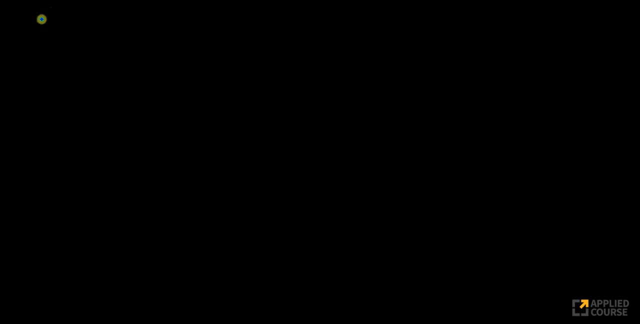 I have given you a high-level overview, but let us go step by step. So the working of a Turing of a UTM, the working of the working, the workings of a UTM, So let us call the UTM. 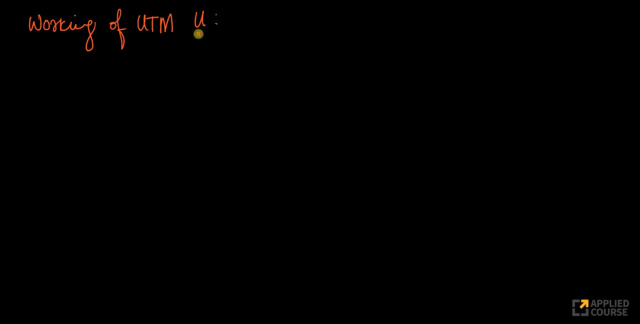 itself as U. We will define the UTM. We will use the term U or the alphabet U to represent a UTM. Now the UTM has three tapes, So let me go one by one. The first tape: let us call this as tape. 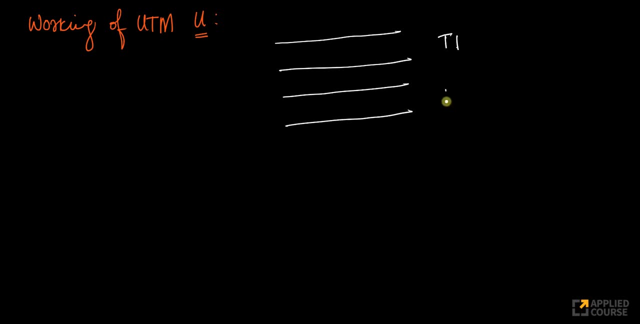 one. It has three tapes. The second tape T2.. The third tape T3.. Because we know, remember, a UTM is also a Turing machine And a multi-tape Turing machine is equal to a single-tape Turing. 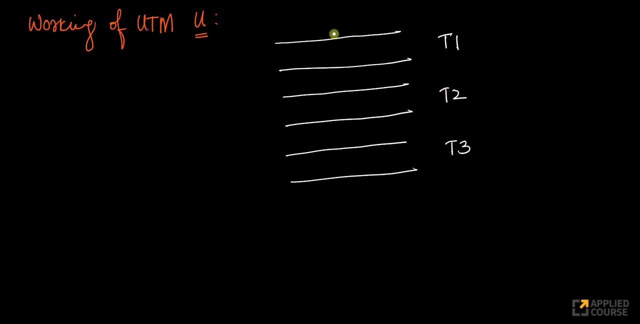 machine. We have discussed about that equality. If I can have a multi-tape Turing machine, I can show that it is equal to a single-tape Turing machine. So the way I will simulate again what is my task here. I have to simulate the working of this Turing machine M, whose code: 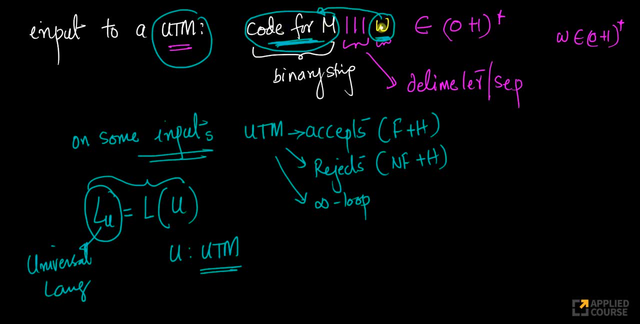 we have on this word W and see if, upon ingesting this word, does this Turing machine reach a final state or not, Does it accept or not. That is all, Basically, that is what we have to determine. So what we will do is step by step, like this: So on this, on tape, one I will actually give. 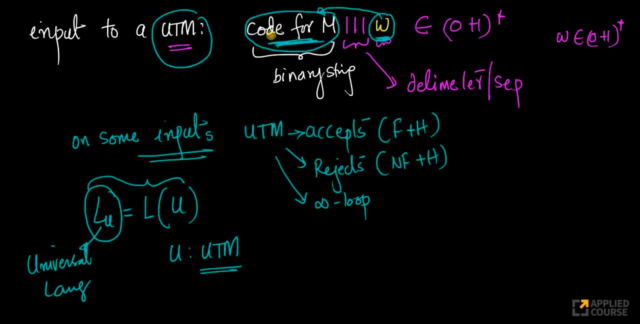 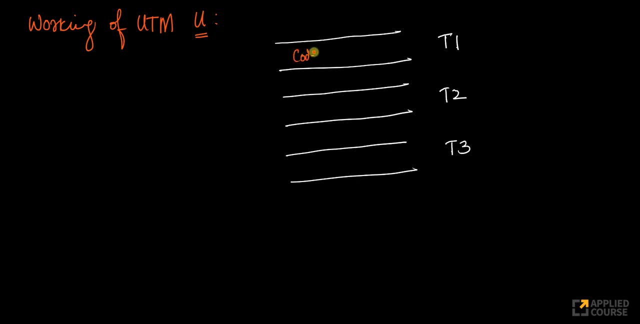 the code. So let us assume M is the code. So let us assume M is the code for your Turing machine. Let me write the whole thing. So the code, the code for M, then delimited by the word itself. This is what I have on my tape one. So my tape one consists of two parts. 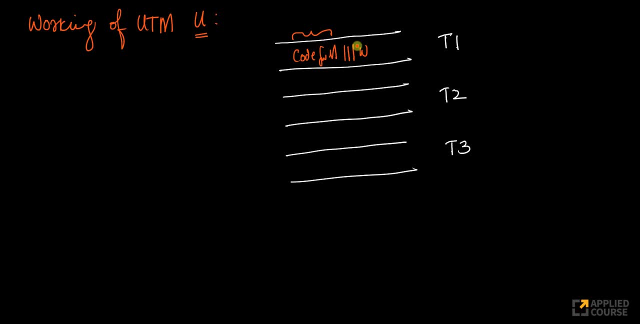 My tape one consists of the code for Turing machine M, three ones as a delimiter and the word itself. That is what my tape one consists of. I will use my tape two as the tape of Turing machine M. Look at this: I have a Turing machine here right M here right. This M also has a tape. 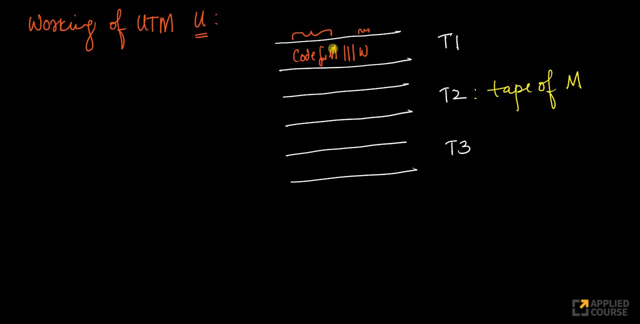 internally This M. look at this If you think about it. if I have to simulate this M, I need to simulate the tape of M, So I will. I will use this tape two to simulate, to simulate the tape of. 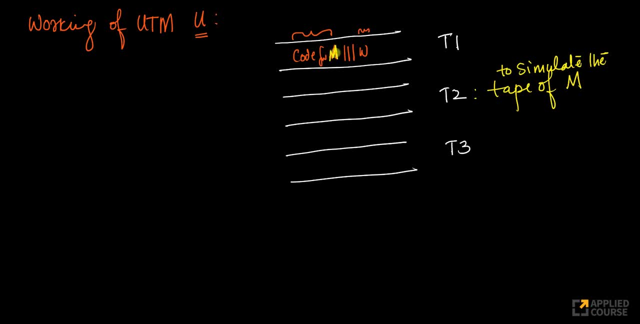 the Turing machine M here. So this, this Turing machine is M. This whole Turing machine is you. T3 itself I will use to store the current state. I will use T3 itself to store the current state, So the current state of of this Turing machine M, while I am simulating the whole thing during. 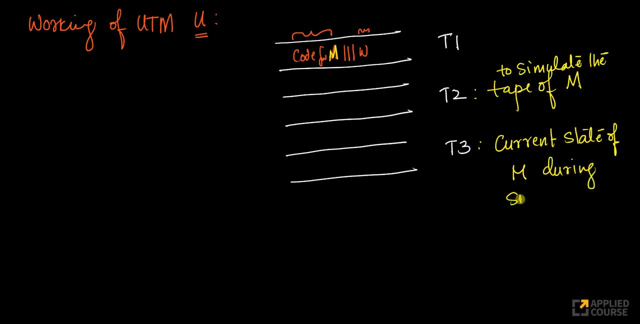 simulation, during simulation. I will explain you how the whole simulation works. It is actually fairly straightforward. Once you see it, it all becomes straightforward, right? Of course, all of them are infinite tapes. Nothing stops us from having infinite tapes here. It is a multi-tape. 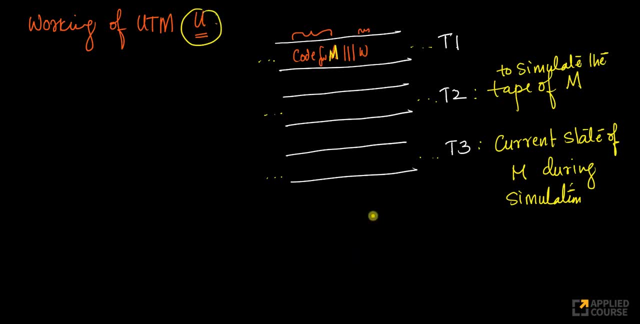 So U itself is a is a three-tape Turing machine, right. So now let us go and understand how, step by step, everything works. The first step that I will do here, the first, the very first step is: first I will check if M is valid code or not. 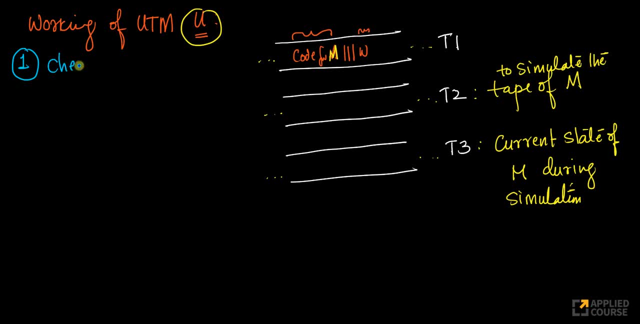 Because very important, right? So check, check, check. if M is valid, If M is a valid Turing machine code, If M is a valid Turing machine code, right? So we can all see I also have a finite control here, right, I have a finite control unit. Let us not forget it For this. 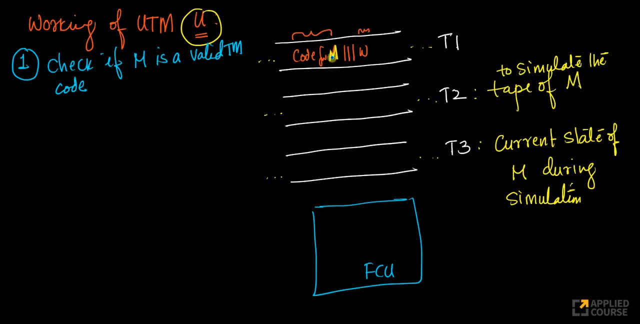 finite control unit. what I will do here is: I- I have a string here. Look at this. I have a. I have a binary string here. This is nothing but a series of zeros and ones right. So this code. 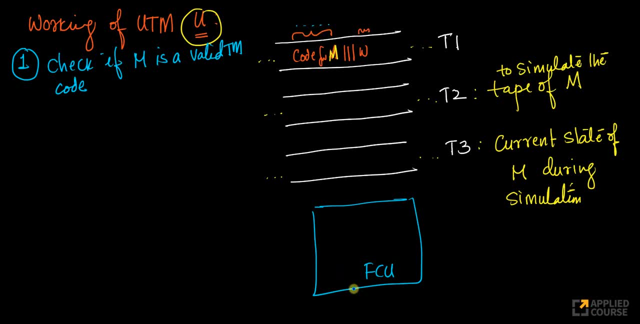 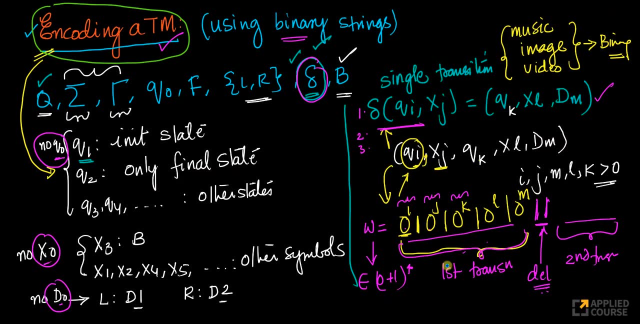 for M. I will start scanning it and I will see if it is a valid Turing machine code or not. So valid Turing machine code should not start with one And it has to have this exact pattern. Look at this. It has to exactly have. it has to exactly have this type of strings, right. It exactly needs. 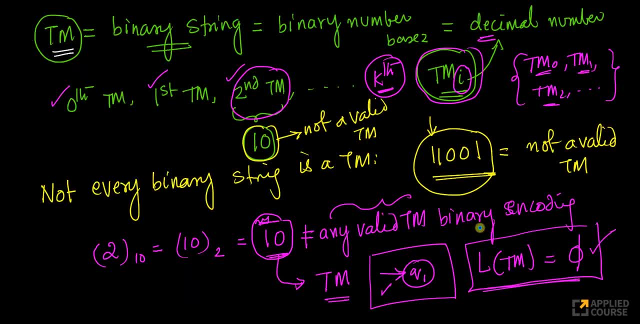 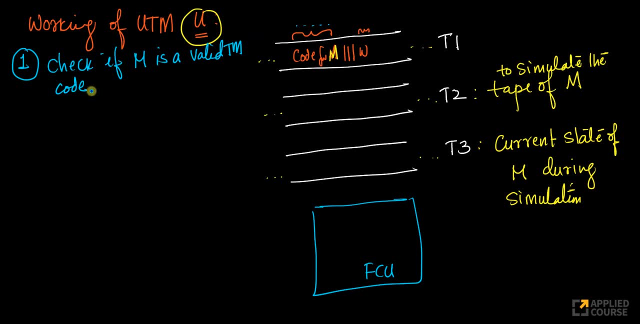 to have this. If it has, if it has strings which are valid, which is very easy to check, right, You can just have a bunch of transitions and check for them The moment you check. this suppose, if it is not okay, Check if M is valid, If not, no. If it is yes, we will continue. If it is no. 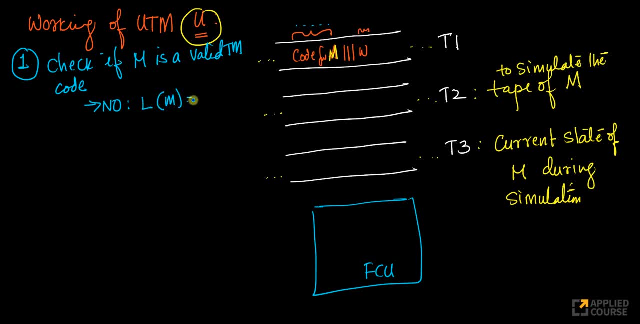 then what do we know? We know that the language accepted by the Turing machine is a null set. We know that, Which means this word will never be accepted by this. which implies: which implies W does not belong to the language accepted by machine. which implies: Then, what should I do? 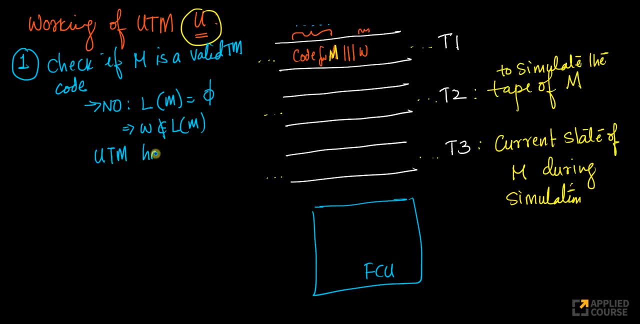 Then the universal Turing machine simply halts and rejects. Halt plus reject: Done Problem solved. First step. First step is a check if M is valid or not. Second step: Let us go to the second step now. Let us assume: yes, Okay, Yes, Continue, Okay, The second option. 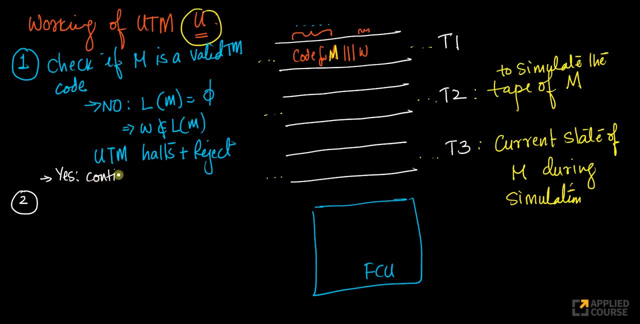 is, yes, it is a valid Turing machine, Then continue. If it is not a valid Turing machine, then again to check whether it is a it is a valid Turing machine or not. I can write some simple transitions in my finite control unit of U itself. See, this whole thing is my U, So 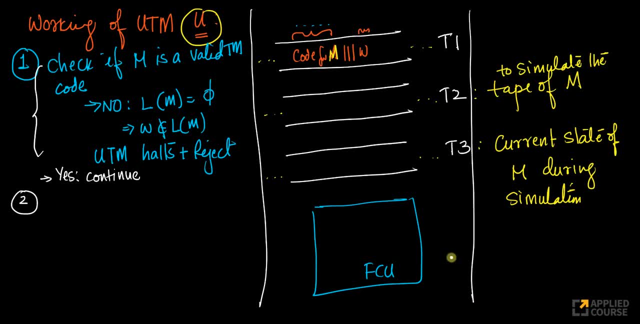 let me draw the boundary box here, right? So this whole thing is my universal Turing machine, U right, Including this FCU, the finite control unit, right? So now comes the second step. What I will do now is: whatever is the, is W, whatever is the input- look at this On T2,. 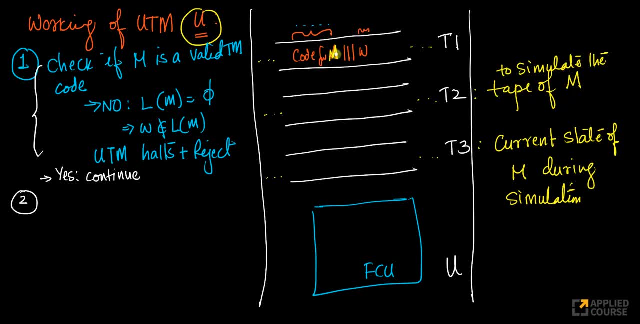 we want to simulate the tape of M. Now, when I am trying to simulate M, imagine M itself is running. Then what happens then? This W will be present on the, on the tape of M. So I will copy W here. 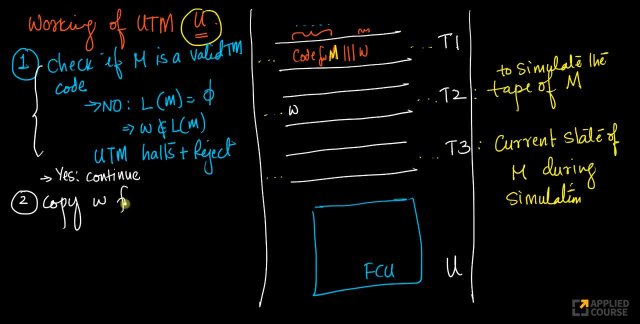 I will copy copy W from from T1 to T2.. And that is very simple. The finite control unit can do that. How does it do that? It keeps scanning this till the time it encounters 3, 1s, The moment it. 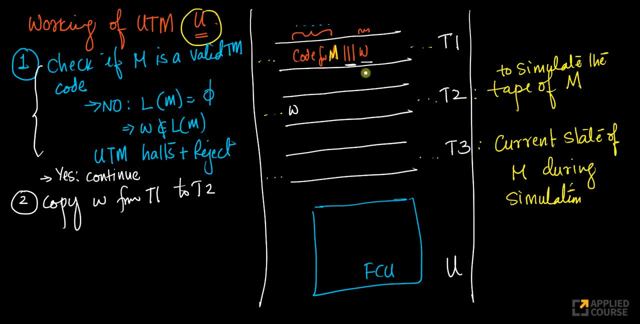 encounters 3 1s, it will keep scanning everything, whatever it sees, because it has 3 heads, right? Look at this: This finite control unit has 3 tapes, which means it has 3 heads. So whatever it reads here, it will write here till the time it encounters a blank. Okay. 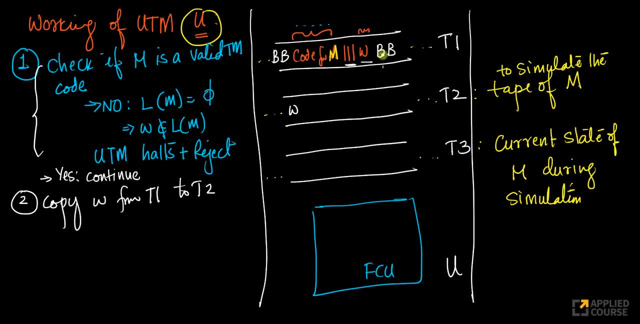 there will be a blank here. So this will be a blank here. So this will be a blank here. So blanks here. right, Obviously, there will be blanks on this step. So till the time it encounters a blank, it will keep copying, it will read from this and it will write to this. We can do that. 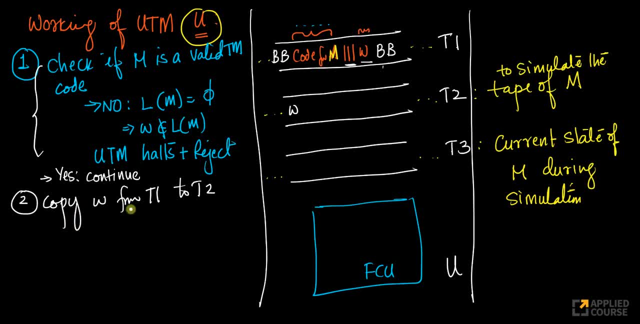 right Because we have three independent read write heads right. So copy w from t1 to t2, second step. Third step, right. Third step: initialize t3,. initialize t3 with the initial state. initialize t3 with initial state of m. What is the initial state of m In the binary? 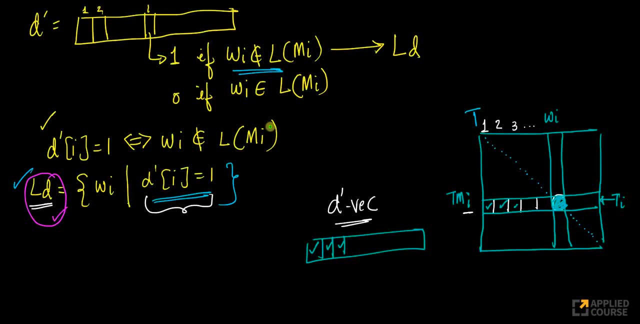 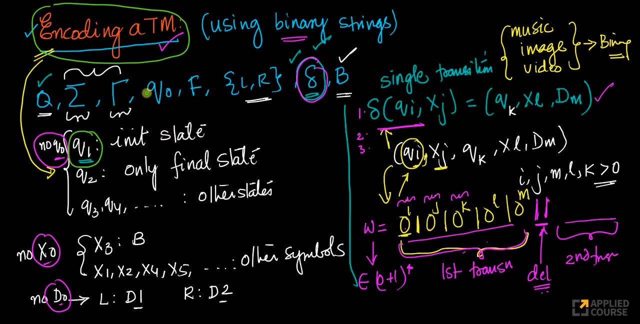 encoding, we said: q1 is always the default initial state. Let us go back there. I will keep going back there. So that see what did we say: q1 is always thought of as the initial state, right? When we did the binary encoding of a tuning machine, right? So let us go back there again now. 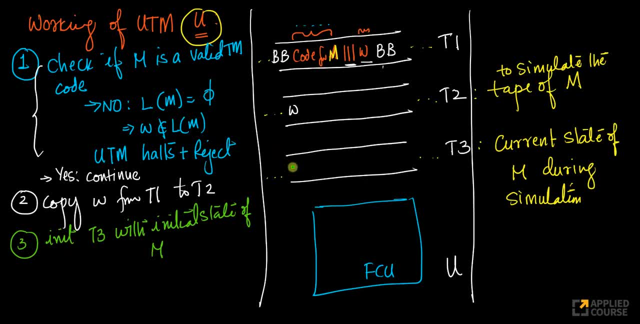 Okay, So what is the initial state? q1,, which means: how do you represent q1 here? You will have blank, blank. This is 1, blank, blank, blank. sorry. 0, not 1, sorry. This 1, 0 basically represents q1, right, And my read. 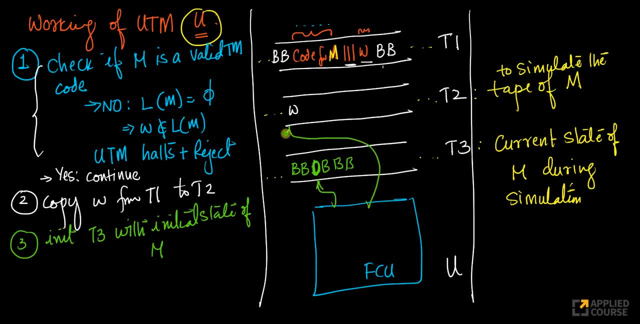 write head is here. Initially, my read write head for this will be here. My read write head will be here. Now I am starting everything right. Very simple code. Three steps First. three steps are done. Next comes the whole simulation part. Next, what do I have to do? Look at this. The next step. 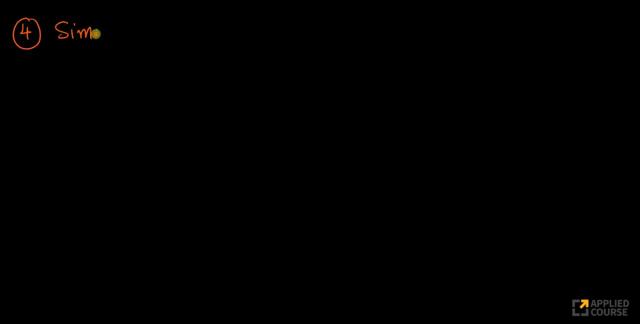 that I have to do is: I have to do a simulation, So I have to do a simulation, So I have to do a simulation. So what do I have to do? The fourth step is: I have to simulate, I have to simulate. 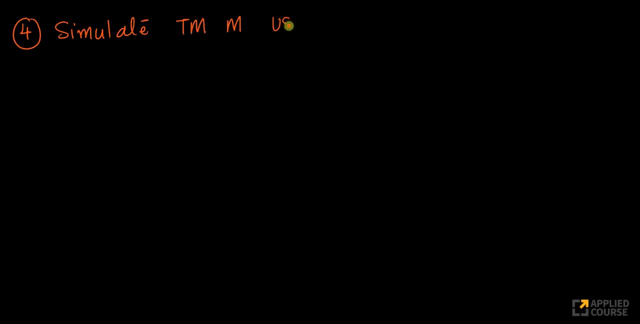 Turing machine M using using tapes T1, T2 and T3.. Okay, Let us see how to do that. It is not rocket science, It is actually simple. So, right now, what is my state right now, My current state? 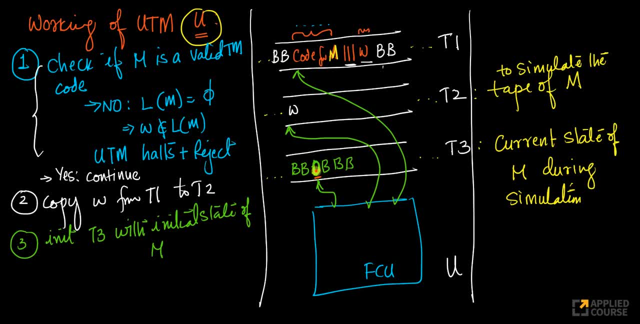 is q1 because there is only 1, 0 here. My current state is q1.. Suppose I have an input word also here. Let us assume my input word Here. we assume all the words belong to 0. So I have to do a. 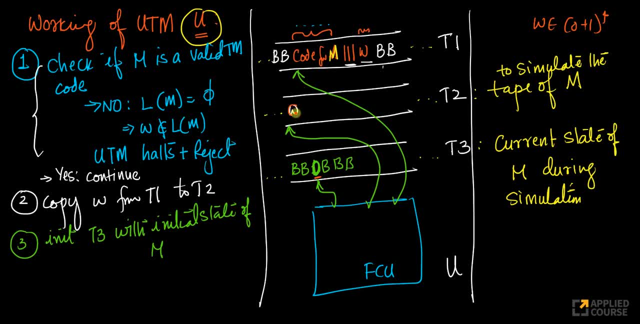 0 plus 1 star. Okay, Just for simplicity, Let us assume my input word is 0011.. Let us just say, for example: Okay, I just wanted to explain this with an example. Then what do I want? 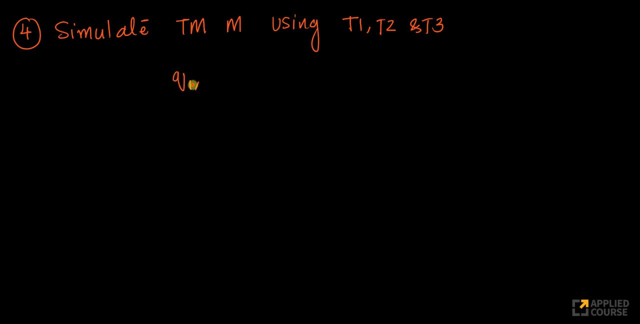 What transition should I look for? My current state is q1.. My current state is q1.. My input is 0. So what is the transition on this Right? That is what I need to obtain now. Now, let us assume. 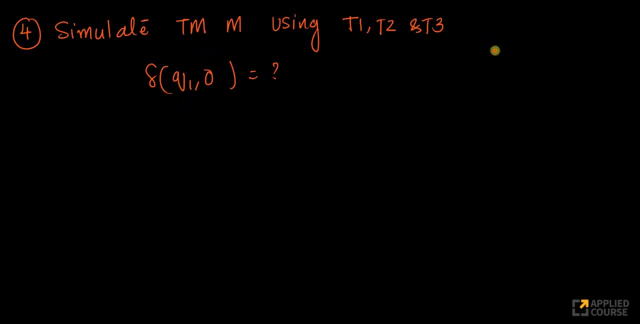 because we have two symbols here. My w consists of 0s and 1s. What are my symbols? x1, x2, x3, if you recall Right, This is what. if you recall the binary encoding of a Turing machine, You can go back. 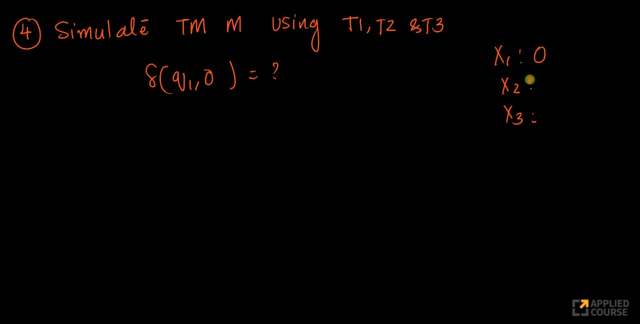 and check that also. So I will assume that 0 is x1, 1 is x2, blank is x3. Then I can write this as: look at this. Then I can write this as x1 on this input. Now, on this input, what is the? 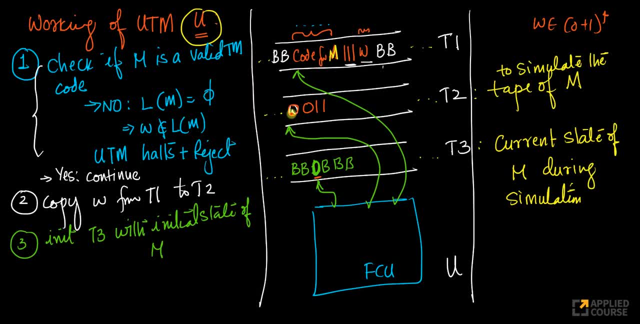 output. I need to find this first, because my input right now, because 0 is nothing but x1.. 0 is x1.. Okay. Next, my state is q1.. Look at this: My state is q1 because there is only: 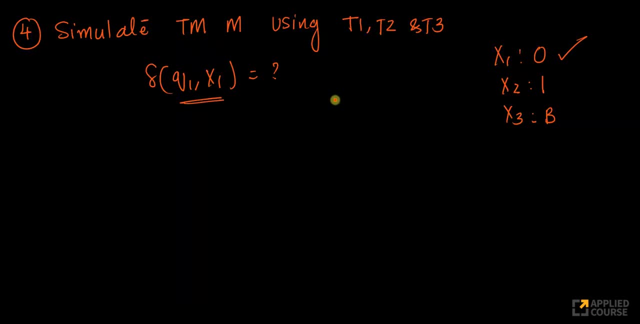 1, 0 here. Now I need to find what is the transition for this. For that there is a code for m. Look at this. There is a code for m. There is a binary code for m, So I will start scanning. 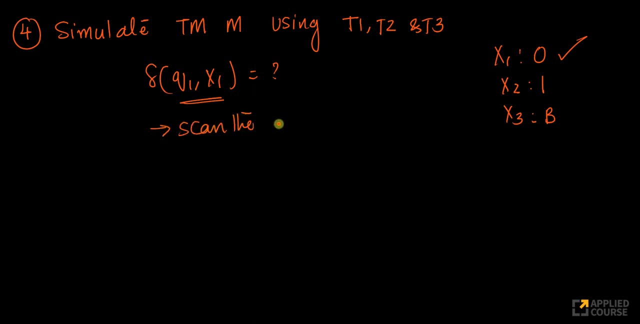 So now what I will do. I will start scan, scan the code for m, Scan the code for m. I keep scanning till the time I get this, because what I want here is a 0 corresponding to q1, a delimiter. 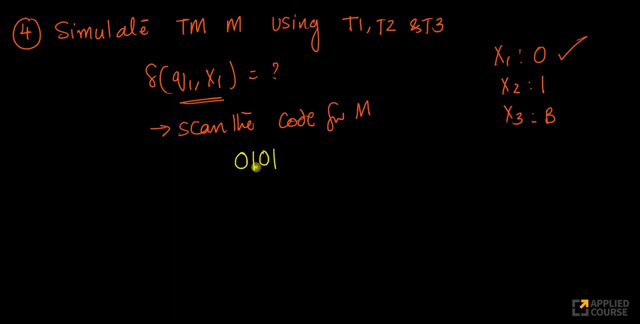 a 0 corresponding to x1.. When I encounter this again, this can either be at the starting or this can be here, which means there is some other transition here. The moment I look for this, the moment I encounter this pattern, I can easily 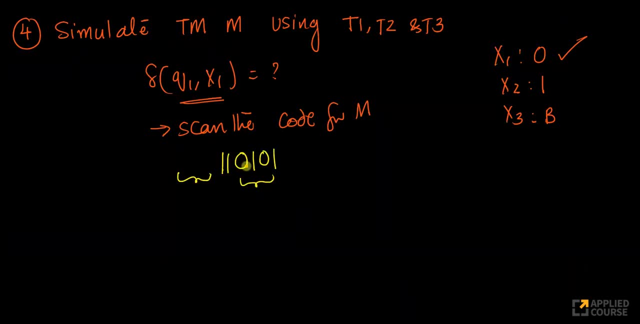 discover this pattern using my finite control unit. The moment I discover this pattern, the moment I discover this: 0, 1, 0, 1,. what does this imply? Look at how we encoded the transitions of the Turing machine m itself. This basically means the transition on q1, x1, because there is 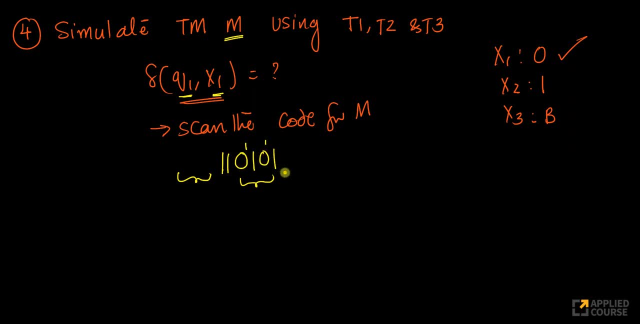 only 1 here. This is 0.. power 1: 0. power 1. right, then let's assume, let's assume here that i have two zeros after this 1, then let's assume i also have two zeros 1, two zeros double 1. so now i'll read this, now what? 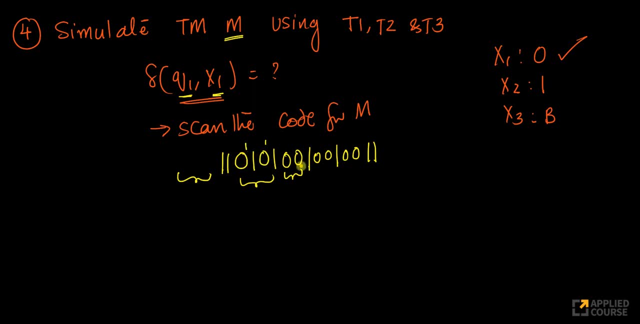 does this? two zeros basically mean? this means, on q1, x1, i should transition to q2. look at this. it says i should transition to q2. right, and instead of x1, my tape symbol should be x2. my tape symbol should be x2. what is x2? x2 is nothing but 1 and i should move right. so this implies right. 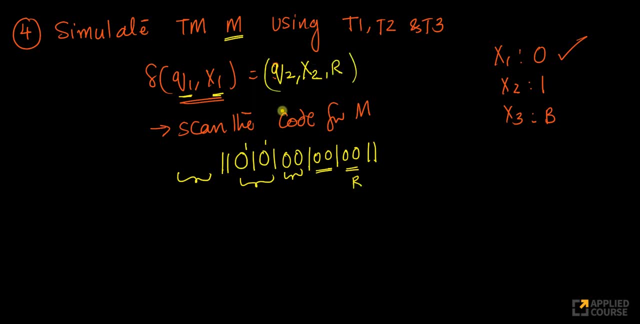 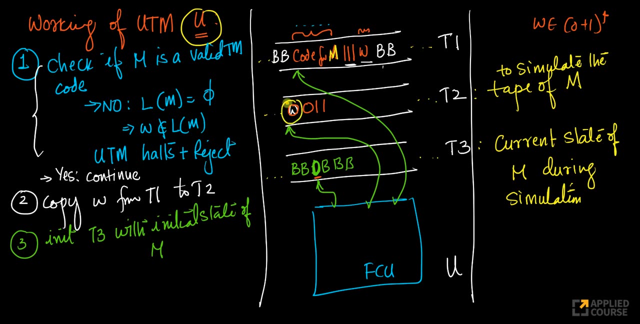 right. this implies right right. so what i've done here is i've scanned the code for m for this transition, because look at this my current symbol, i have here my current state, i have here right. based on these two, i'll start looking for this code here. i would start looking. 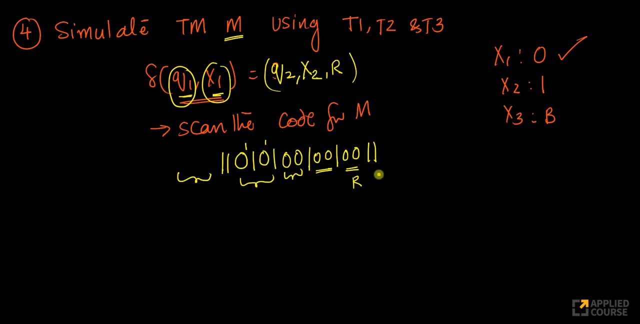 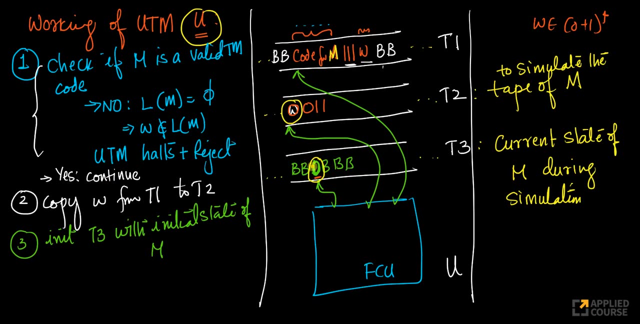 for the code on my turing machine m. so the moment i find this, i know where i need to transition. my next state is q1- q2. the moment my next state is q2. what i'll do here. what i'll do here is: i want to jump from. 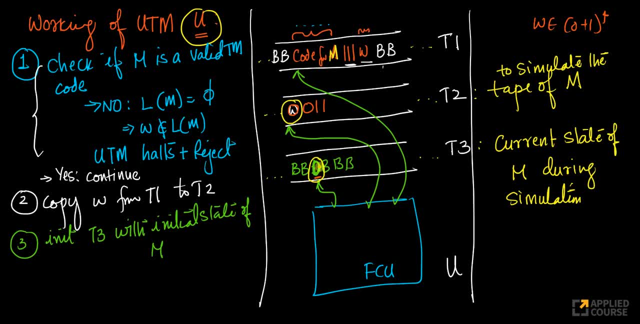 q. this is q1, right, because there is only one zero. i want to jump to q2, which means i'll edit this to have two zeros the moment it has two zeros. what does this mean? this means my current state is q2, right? i'm simulating my state here. look at this. i'm keeping track of my states here. number one: 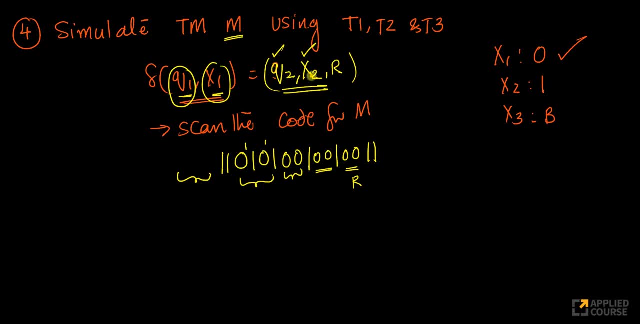 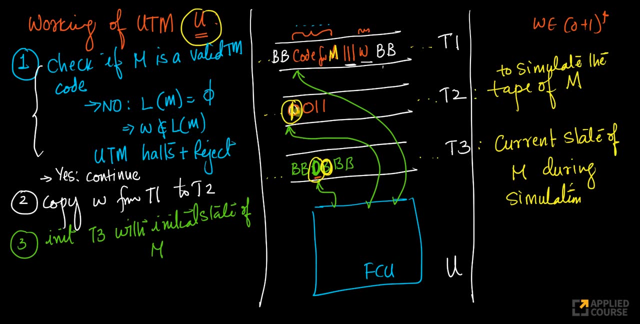 then my input has to be changed to 1, because x2 equals to 1. right, so what i'll do here? i'll change this 0 to 1. look at this: because i have two zeros, I have these read write heads. I can change each of them independently. right next I have to move. 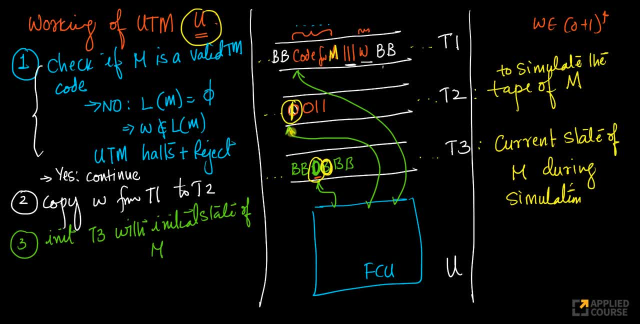 right. so what does this say? I have to move right, so I will simply move right. my read write head now will move right. my read write head now will move right right. next, what do I have next? my state is again again. I again scan for it. next, what is my state? q2 on 1 right, q2 on what is? what is my? 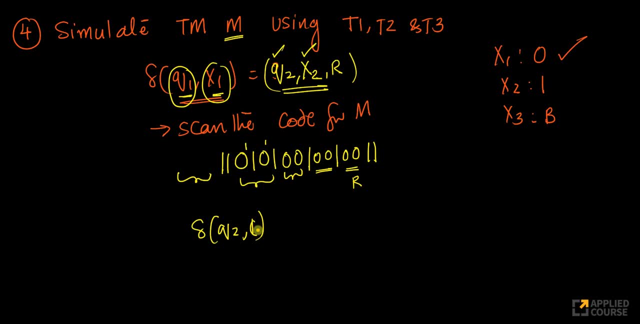 input now. my input now is 0. sorry, my input now is again 0. q2 on 0. what is 0? 0 is nothing but x1. right, 0 is nothing but x1. now, what is? how do I find what this transition should be now? I should. 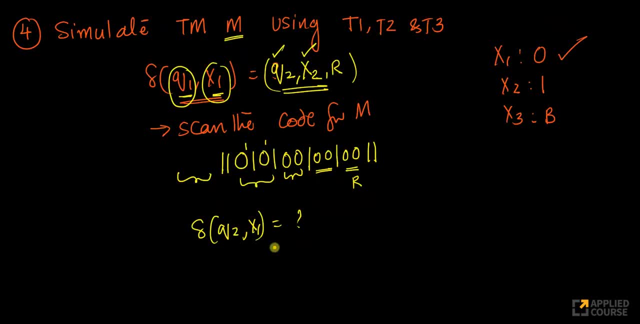 again scan the. I should again scan the code here and I should look for some, so some, some other transition here. then q2: what is q2? two zeros x1, so this, so this whole thing corresponds to q2 x1. then I will get something else again. so the. 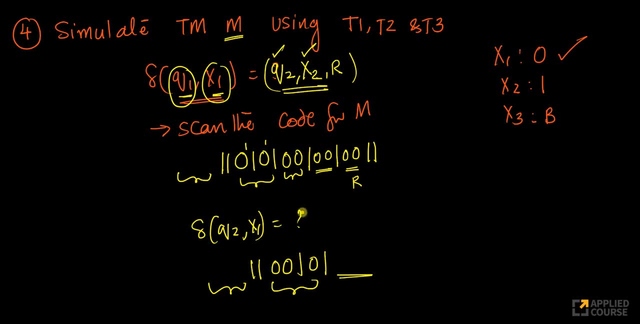 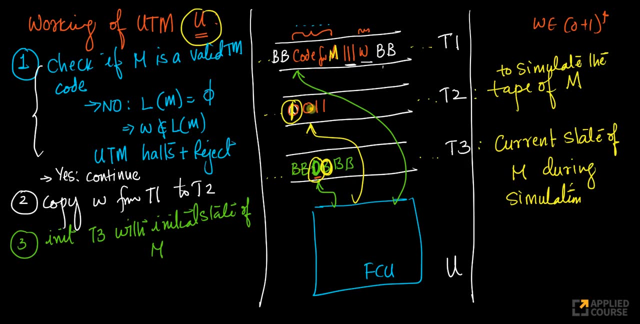 you, I'll get some other transition right. so let's assume this transition to some other state changes x1 to something right or left right. so based on that, again, just like the way we have done in the previous step, I'll change the state, I'll replace this and I'll keep doing it. I can. 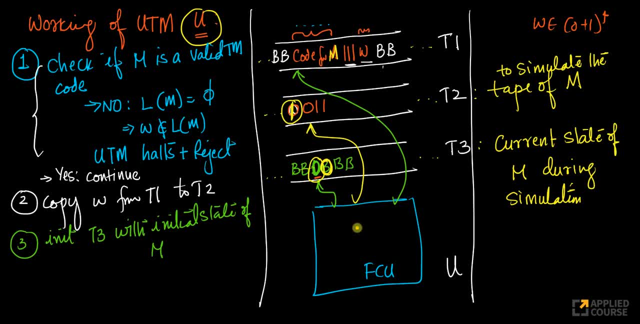 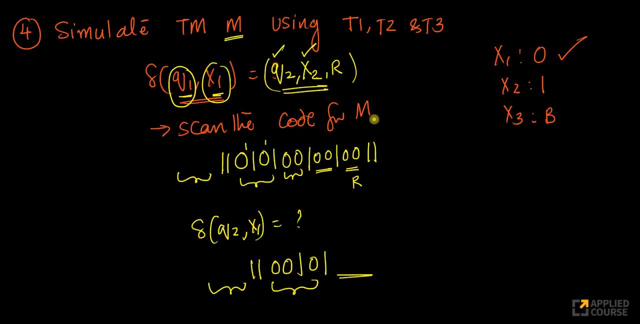 keep doing this. look at this. I keep doing the same thing till the time I reach a final state or till the time I have exhausted the whole input right now, the way, the way UTM now accepts or rejects as follows. look at this: now I've simulated the whole thing right. so step 5: I'm simulating. 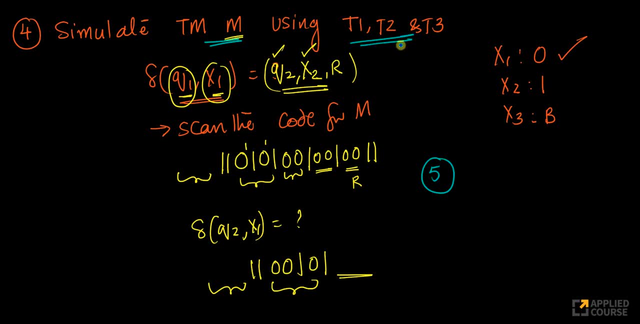 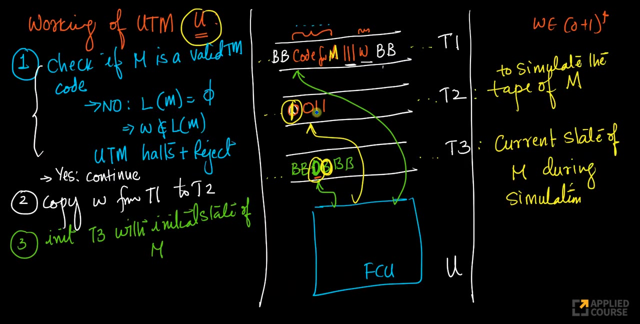 the whole Turing machine M using these three tips, right, and we've seen how to simulate it. it's very simple: now, if M accepts, now if M accepts, if M accepts W, which means? what does that mean? it means, but by reading w, by reading w, if I reach a final state, I know. 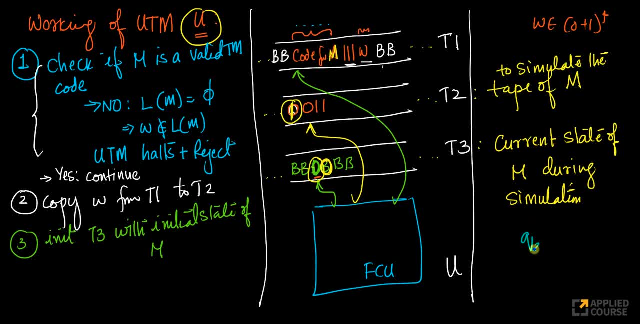 what the final state here? right, the final state always by default. the final state is q2. we already talked about it by default in in the binary encoding. the final state is q2, then you, the initial state is Q1, right? So if I have reached a final state and if I have halted, 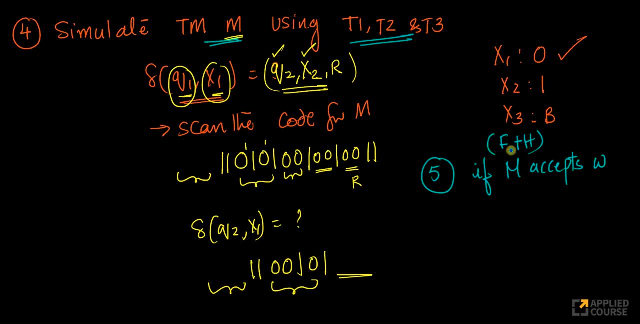 so final state plus halt. So by reading or while reading W, if I reach a final state and if I halt, then M accepts W. right, And I can easily decipher that right. How do I know that I have halted? 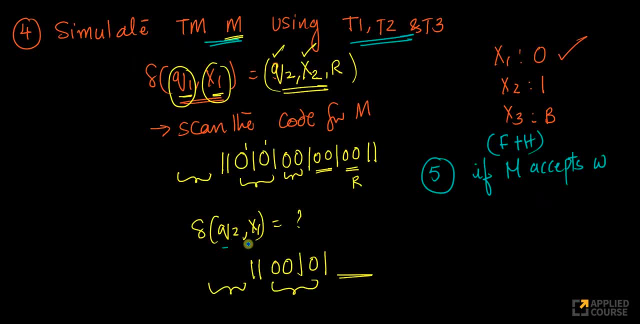 If I do not have any other transitions. if, for example, for something like this, if no transition is defined right, then I know that I am halting there. I cannot do anything from there, So I have halted. and if the state that I am currently in is a final state, 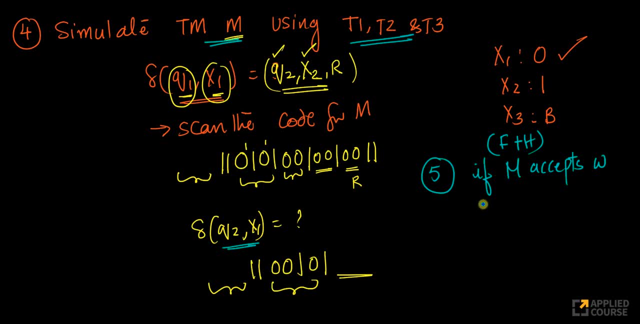 then M accepts W and UTM can easily detect it. Then the UTM, the universal Turing machine, also accepts. the Turing machine also accepts the input. What is the input here? The code for M. So let me write this down below here: So the UTM also accepts the. 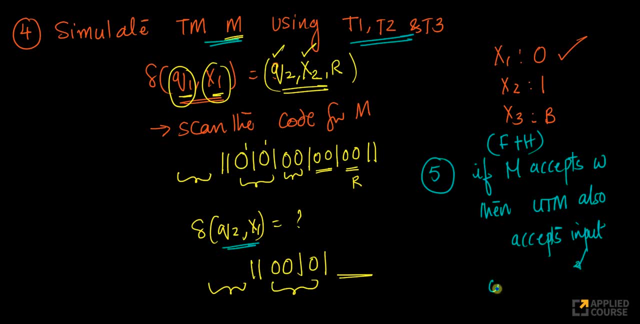 input. What is the input for the UTM? The input for the UTM is the code for Turing machine M111 W. Look at this So we know when the Turing, so when M, accepts W, which means through this simulation. 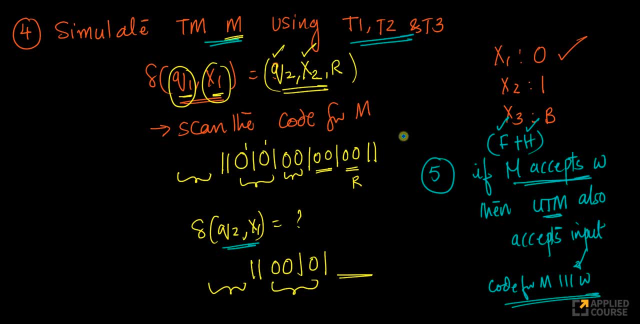 if I reach a final state and if I have halted while I am performing the simulation, then the UTM also says: yes, we have reached a final state. and I know we have reached a final state because Q2 is the only final state and we have halted because there is no transition defined. 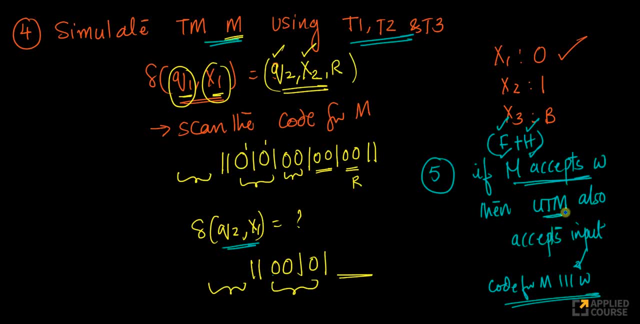 in my whole set of transitions. So I have halted, So I have halted, So I have halted. So in the code for M, once I do that, it says I am also going to accept it. Simply speaking. 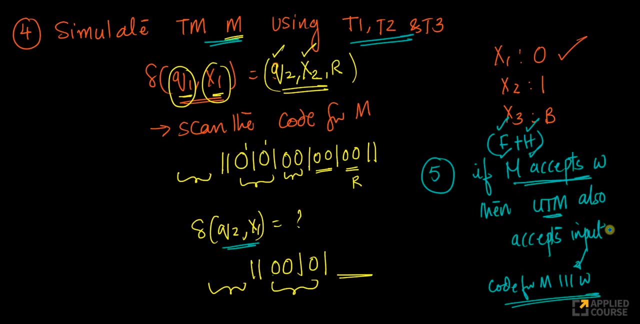 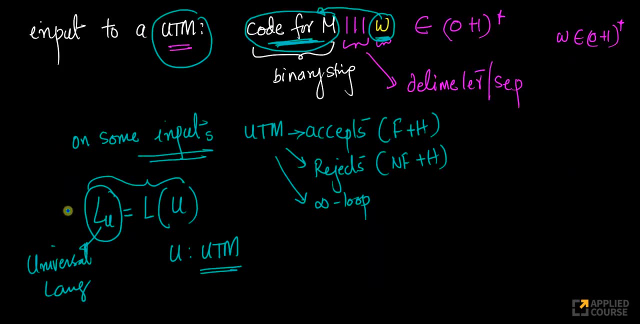 that is what it does. That is what it does in a nutshell. Very simple concept here. So I hope you have understood how a universal Turing machine works- very importantly- and LU itself, because this is a very, very important language. LU is a set of input strings to the universal.